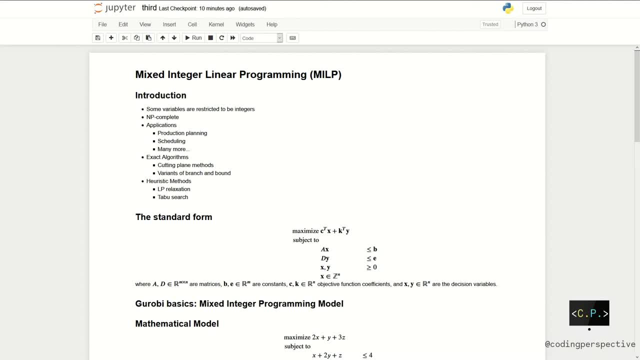 linear programming problems. One class of algorithms are cutting plane methods, which work by solving the LP relaxation, then adding linear constraints that drive the solving of the solution towards being integer without excluding any integer feasible points. Another class of algorithms are variants of the branch-and-bound methods, For example the branch-and-cut. 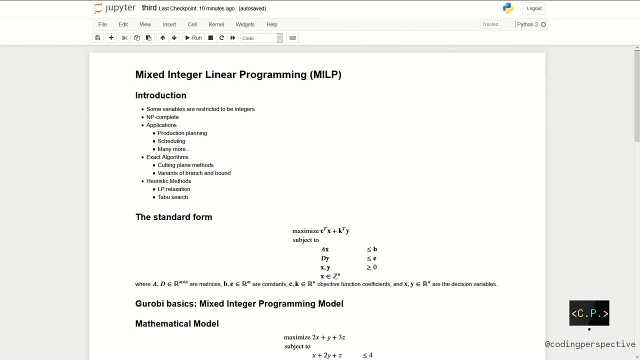 method that combines both branch-and-bound and cutting plane methods. Branch-and-bound algorithms have a number of advantages over algorithms. First, the algorithm can be terminated early and as long as at least one integral solution has been found, the solution can be returned. And there are also many heuristic methods. 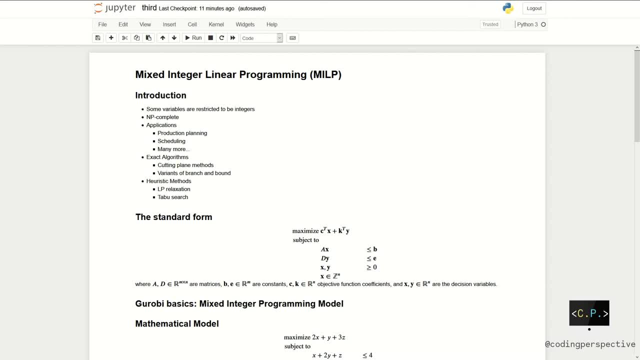 The naive way to solve an MILP is to simply remove the constraints that the algorithm has created and solve the corresponding LP, which is called as the LP relaxation of the program, then round the entries of the solution to the LP relaxation. But not only may the 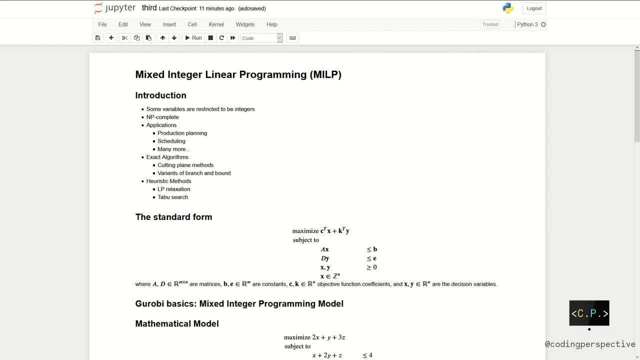 solution not be optimal or it may not even be feasible, that is, it may violate some of the constraints. Tabu search can be used to search for solutions to MILPs. To use tabu search to solve MILPs, moves can be defined as incrementing or decrementing an integer constraint variable of a feasible. 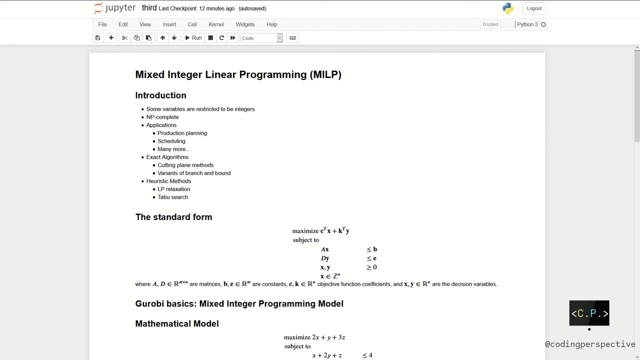 solution while keeping all other integer constraint variables constant, And the unrestricted variables are then solved for. The short-term memory can consist of previously tried solutions, while medium-term memory can consist of values for the integer constraint variables that have resulted in better objective values. Finally, 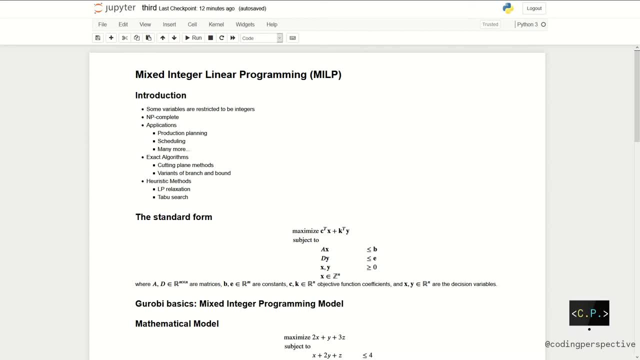 the long-term, can guide the search towards integer values that have not previously been tried. So the standard or canonical form of the ILP's are the following: Maximize or minimize C, x plus K, y subject to A x less than or equal to b, D, y, less than. 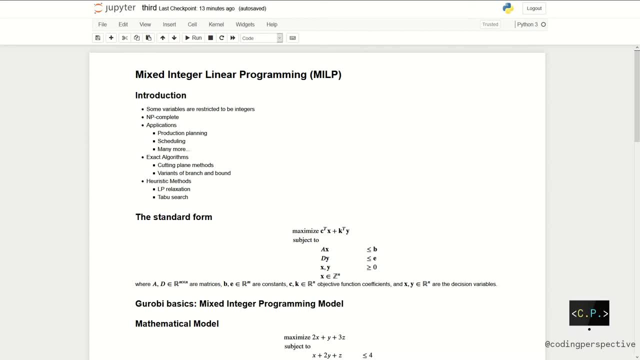 or equal to e, And we have boundary constraints, which are x greater than or equal to 0, y greater than or equal to 0.. Lastly, we have the Integrality constraint on X, So X needs to be an integer. 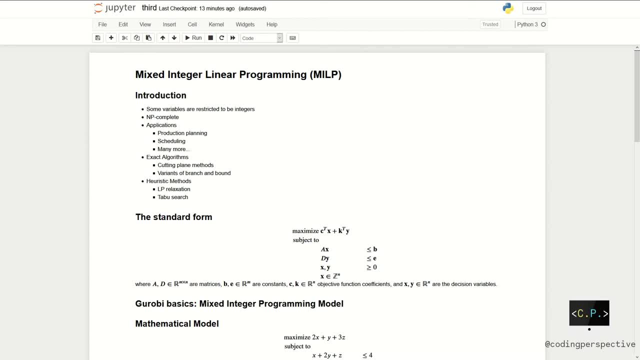 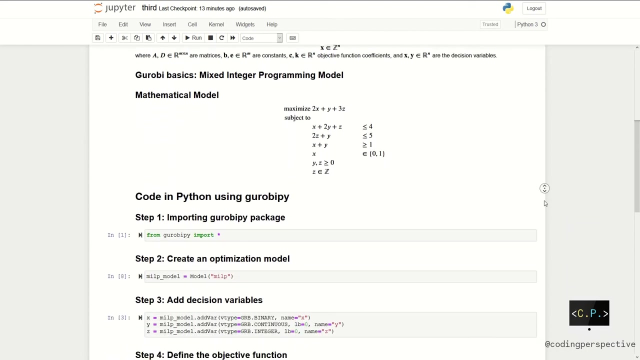 In this problem, a and d are the matrices and b and e are the constraint constants, and c and k are the objective function coefficients, and we are trying to determine the best decision variables, which are x and y. Let us move on. coding an instance of an MILP on Python. 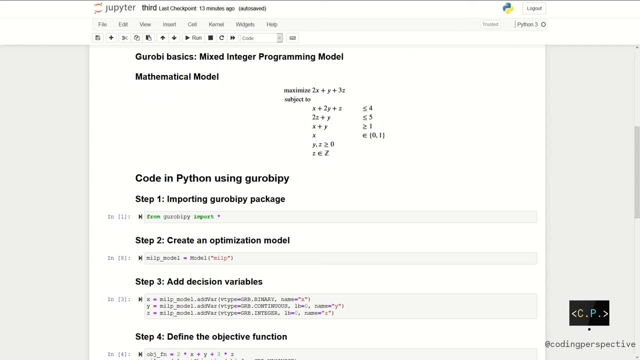 Consider the following maximization problem. We are trying to maximize 2x plus y plus 3z, subject to the constraints. First constraint is x plus 2y plus z less than or equal to 4.. The second one is 2z. 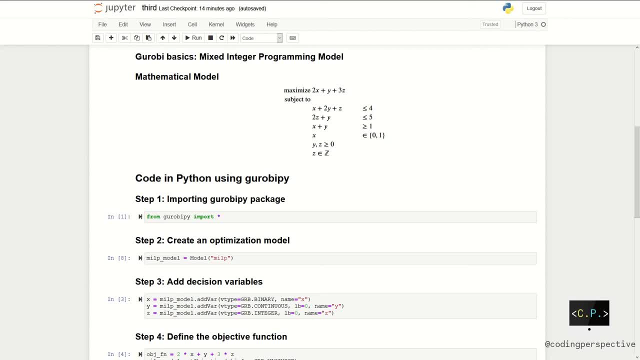 plus y less than or equal to 5. and the last one is x plus y greater than or equal to 4.. Suppose that the decision variable x is binary, z is an integer and y is a continuous variable For the coding part, as you remember from our 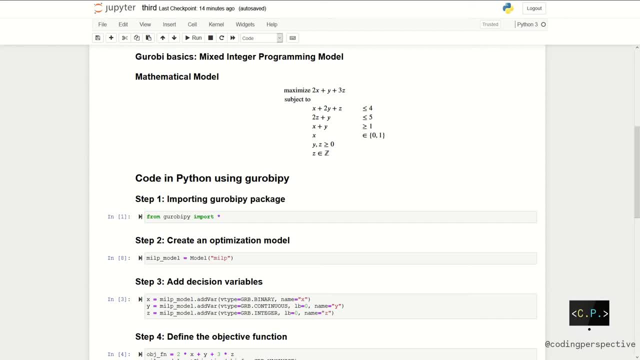 previous video. we first need to import GroovyPy package. In the next step we create our model instance and name it MILP. In step 3, we are going to add decision variables. Again, x is a binary, y is a continuous. 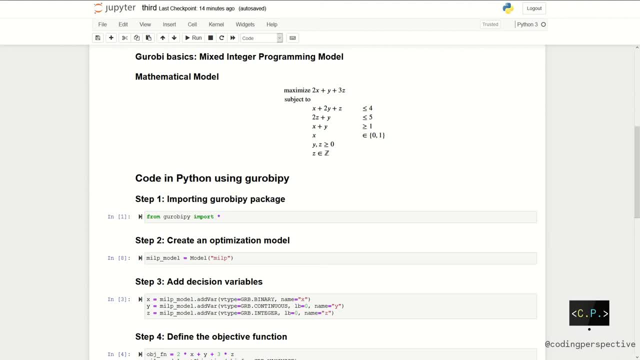 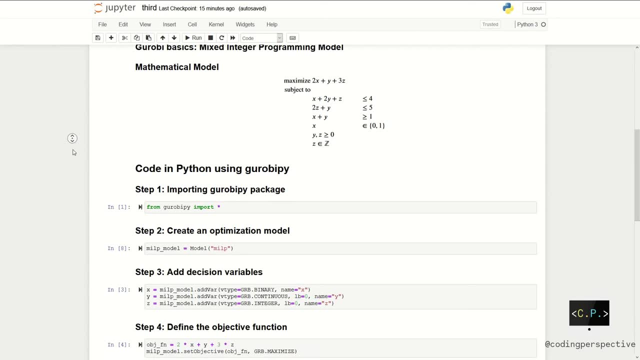 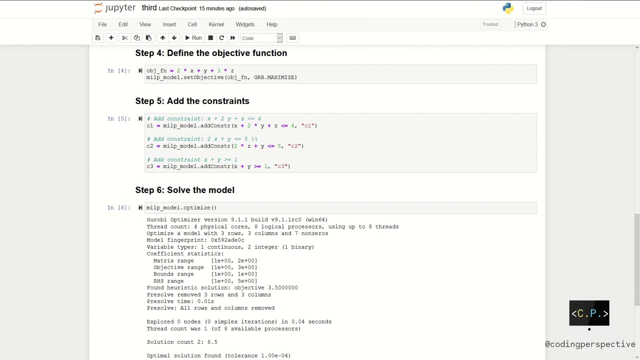 and z is an integer decision variables. We should not forget to add the lower bounds for y and z. We add the decision variables, then we can define our objective function, which is 2x plus y plus 3z. Remember that we want to maximize the objective function. 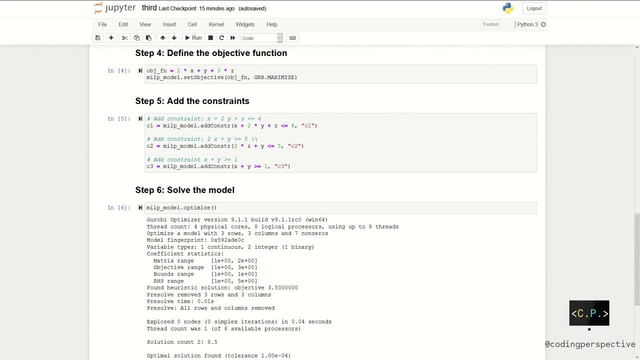 We set the objective function and the aim as maximization. Then we move to the adding constraints. We already add the boundary and integrality constraints when we define the decision variables in step 3.. Now we have three more constraints. First, x plus 2y plus. 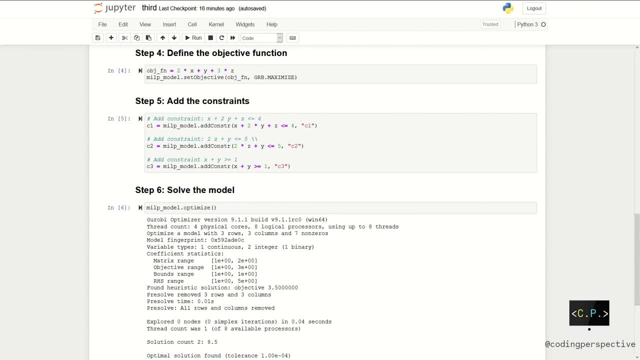 z less than or equal to 4.. Second, 2z plus y less than or equal to 5. And the last: x plus y greater than or equal to 1. We add constraints, we define objective function and then we define also our aim. 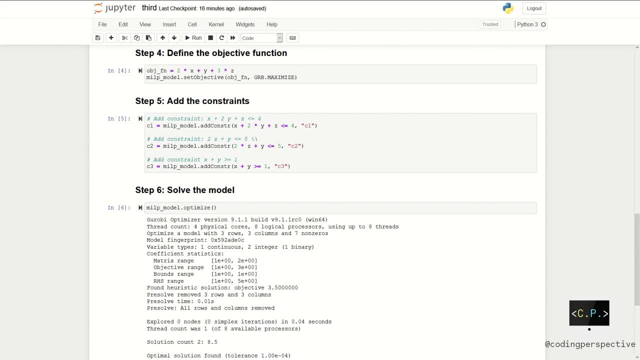 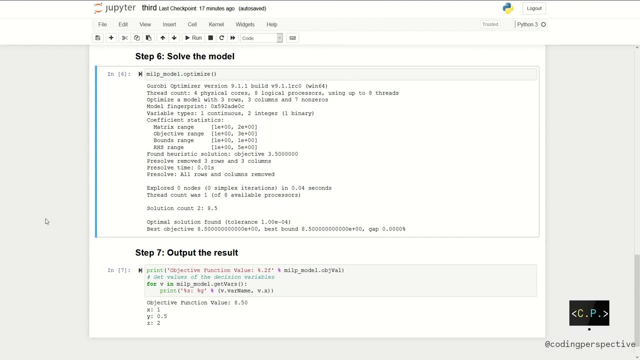 as maximization. Then we can move to solving the model. Now our model is ready to be solved. We will use the function optimize. When we call the function, it evaluates the model and, as you see, it shows that we have two integer variables where one of them is binary. 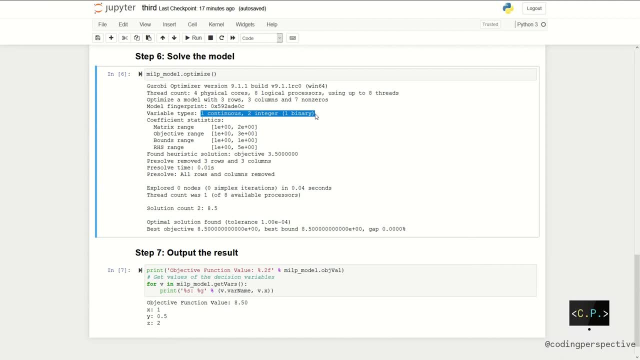 and one continuous variable and it also says that optimal solution is found And it also shows the best objective function value. Let's have a look at the results and the values of the decision variables. We again use the same loop to see all variables When we run the. 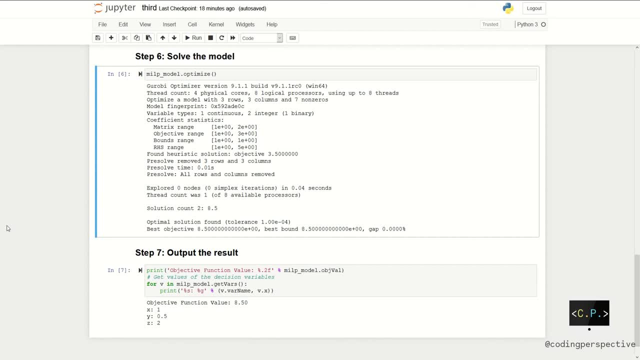 code snippet. under step 7, we see the optimal objective function value, which is 8.5, and optimal decision variable values, which are equal to 1, y equal to 0.5 and z equal to 2.. We have briefly discussed mixed integer linear.